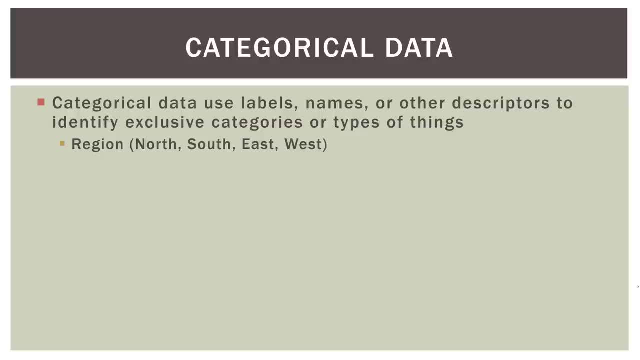 country, state or territory. So common ones are north, south, east or west. Now you could have northeast, southwest or so forth. But let's say you have a office or a factory and you want to label where it's at Now. in this case it cannot be in both north and east the way these categories 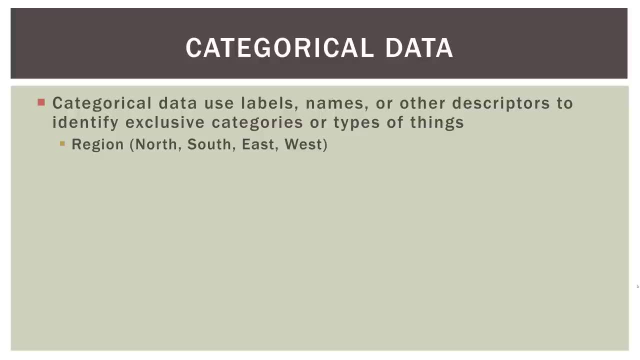 are set up, You'd have to create a different category called northeast. So that's what we mean by exclusive. How about a machine and a factory? So we could have machine one, machine two, machine three and machine four and machine five and machine six. Now let's go back to the 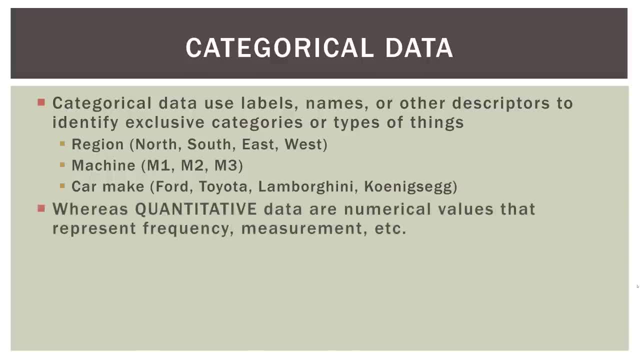 question: Which one do I want to make? So a Ford, a Toyota, a Lamborghini or, my favorite, a Koenigsegg? Now I'm sure you've also heard about quantitative data. So quantitative data in comparison to categorical data are numerical values that represent frequency measurement or 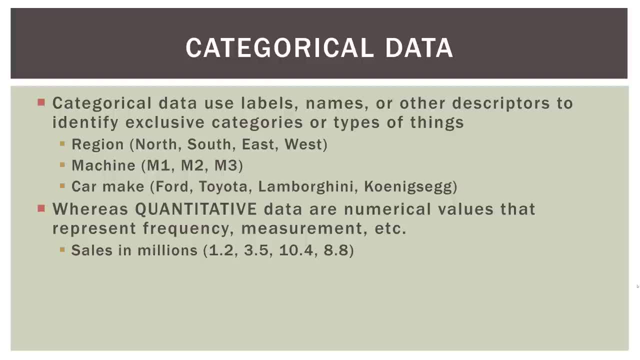 something else like that. So let's look at our regions up above, So we have the region of north, south, east or west and we could have a quantitative data point for sales for those regions. So maybe 1.2 million. 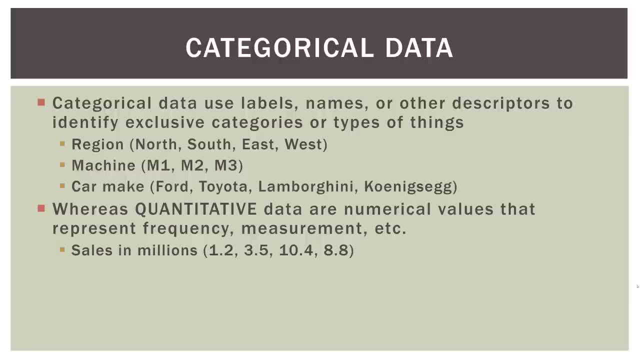 $1.2 million for north, 3.5 million for south, 10.4 for east and 8.8 million for west, for example. So the three machines above could have production units 983,, 1085, and 899.. 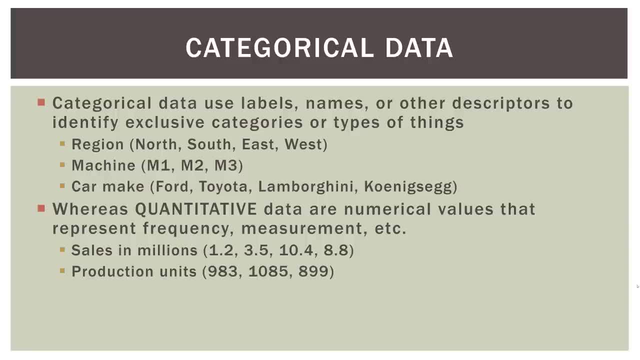 Now it's important to point out that again, those quantitative values go with exclusive categories above, Or we could have the fastest car in miles per hour. So the fastest Ford, which is the Ford GT, will go 216 miles an hour. 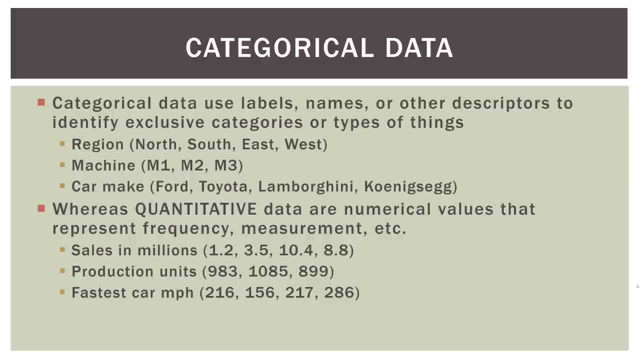 The fastest Toyota ever made, which I believe is the Supra Twin Turbo- I'm a car person, if you can't tell- is 156.. The Lamborghini Aventador will go 217 miles an hour And the Koenigsegg Agera R or RS. 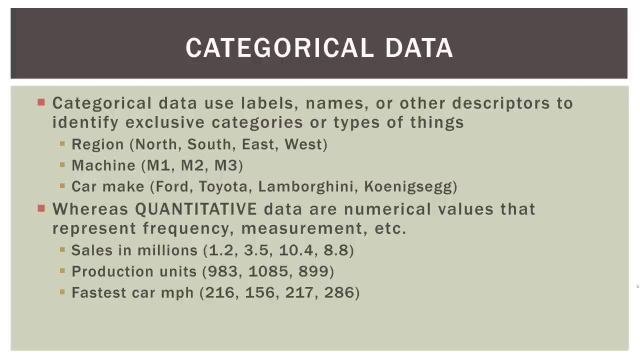 just set a record for 286 miles per hour here in the US, So you can see that we have categories above that are exclusive. that are what we're talking about in this video, and then later we'll talk about more about quantitative data, which are numerical values. 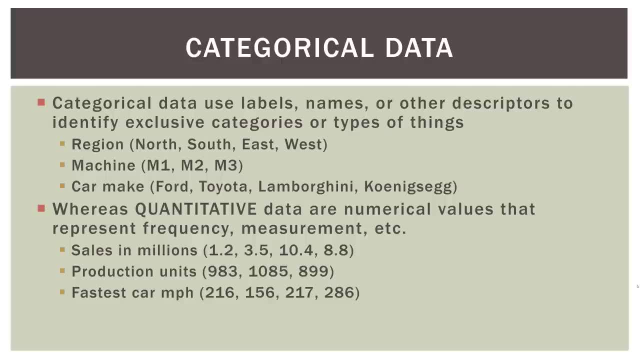 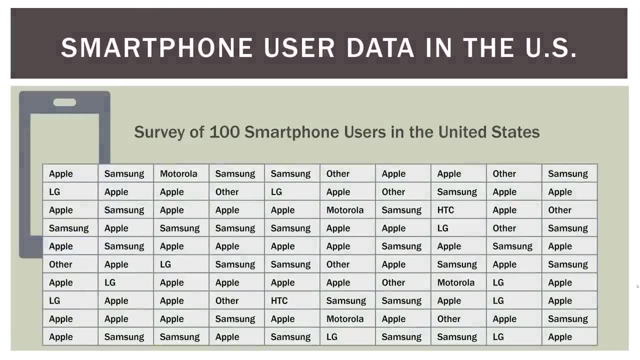 So just fundamental to understand the difference between the two types of data as we move forward. So here are some fake data about smartphone users in the United States. So let's say we did a fictitious study of 100 smartphone users in the US. 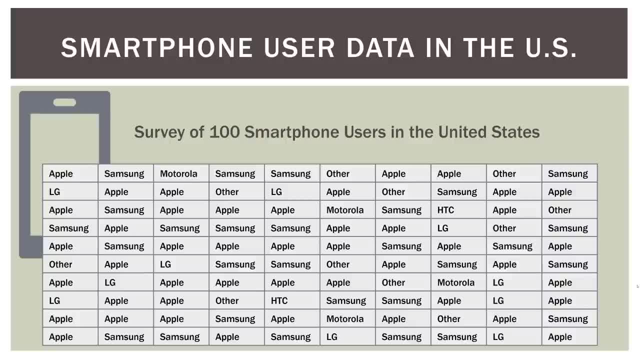 and we asked them: you know who made your primary smartphone? Because sometimes people have more than one. Let's just say your primary smartphone And this is what we have. So we have a mix of Apple, Samsung, LG, other kind of captures, everything else, and Motorola. 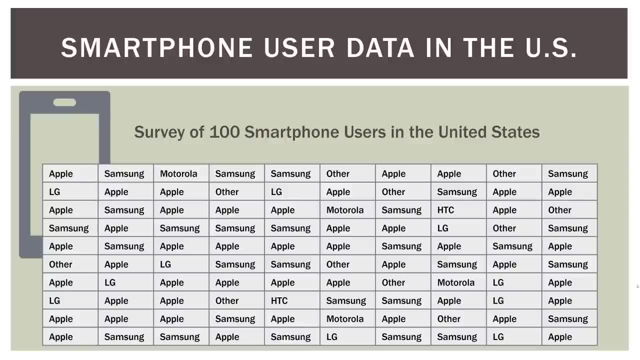 And this is actually approximately the distribution of cell phone makes here in the US. So here is our data. Now the question for this video is: how do we make sense of this? This is just a bunch of rectangles with brands in them or makes of phones in them. 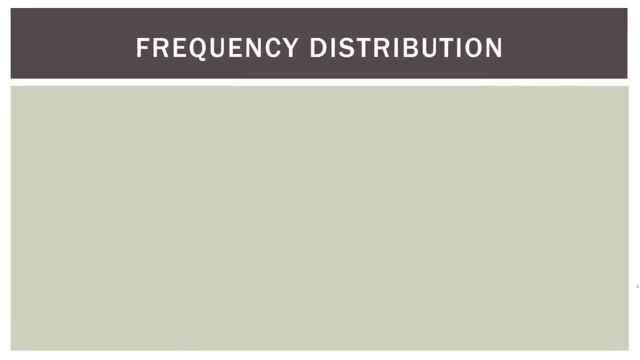 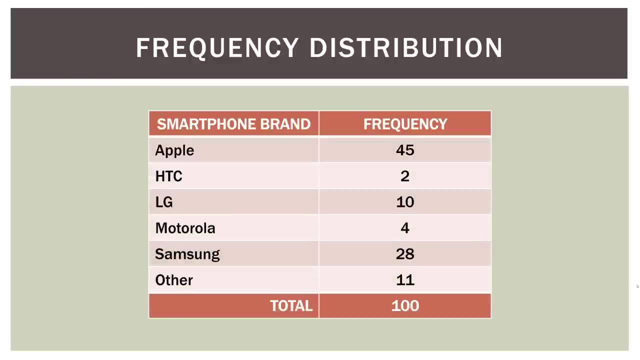 So let's make some sense of it. So the first thing we could do- and it's very simple to do- is create what's called a frequency distribution. Another way of saying that is: we just count them, So we'll go back to our data we had in the previous slide. 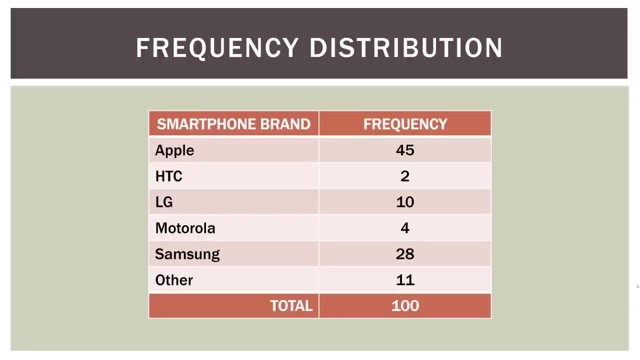 and we just count how many people had Apple phones. There were 45.. HTC were two, LG 10,, Motorola four, Samsung 28, and other mix of brands 11.. Now, as we said, we had 100 observations on the previous slide. 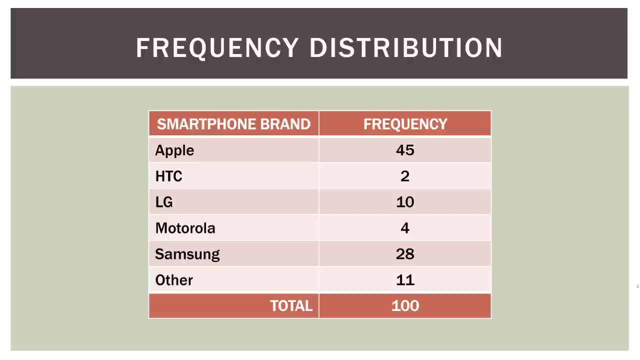 So when we add up our frequencies, it better add up to 100, or we made something else, We made some type of error. So you have to check your frequencies and your totals to make sure they add up to how many observations you had. 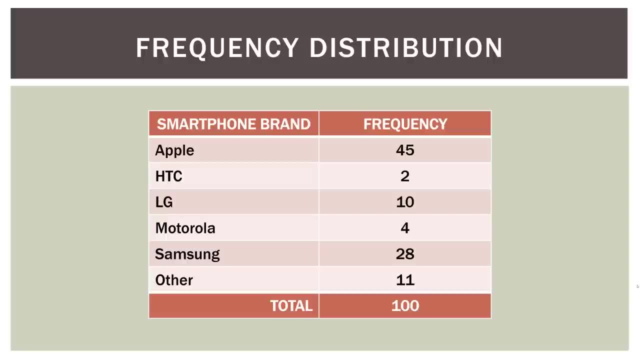 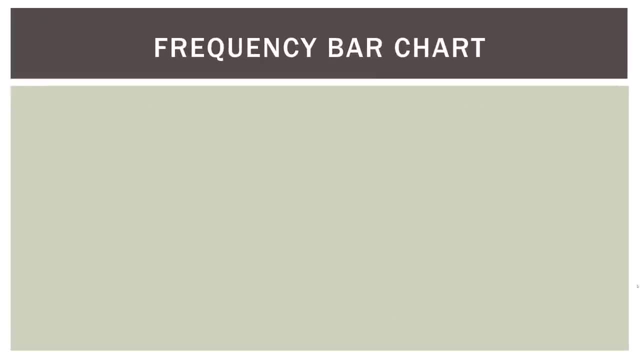 But again, this is very simple: Count it up and write the frequency over in the right-hand column. Now what we can do to visualize this is to make a frequency bar chart, Again, not all that complicated. So here along the bottom, which is our x-axis, 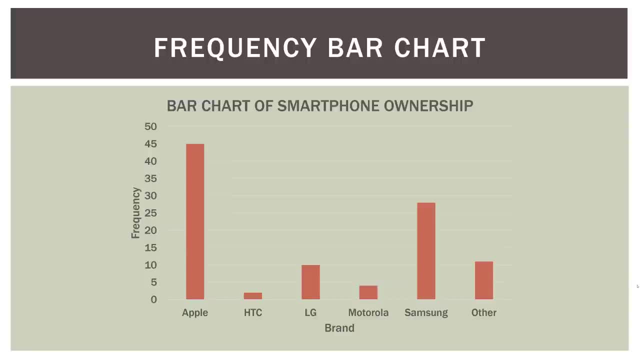 we have the brand of phone: Apple, HTC, et cetera. Over here on the left, on the y-axis, we have the frequency, And then all we do is create a simple bar chart so we can visualize the distribution of phones among these brands. 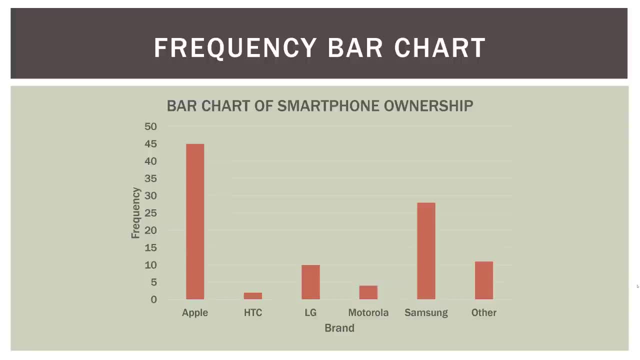 Now I do want to caution you here that you've probably heard of something else called a histogram, and it looks very similar to a bar chart. Now there are some differences. A histogram is for quantitative data. The charts look different. On a histogram, there is no space between the bars. 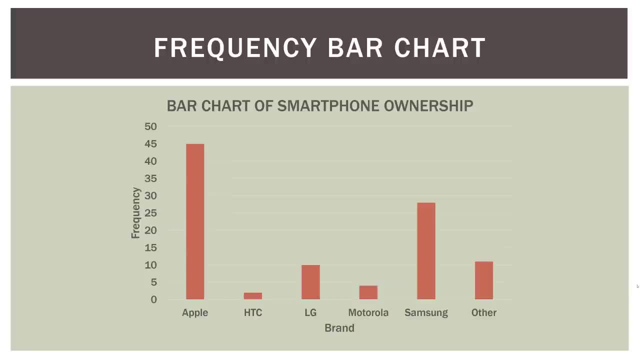 So what all we're doing here is a basic bar chart where we're counting up the frequency of each phone with space between the bars, and then counting up the frequency of the phone, and you can do that in Excel or any other stats program. 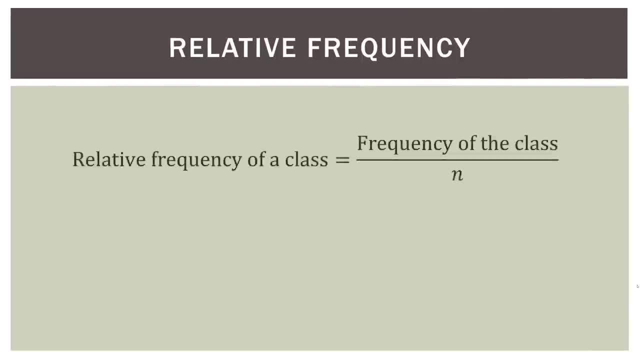 Now we can also talk about another measure called the relative frequency, And again it's not all that difficult. So the relative frequency of a class, which is sort of a part of the category, is the frequency of that occurring over all of our observations. 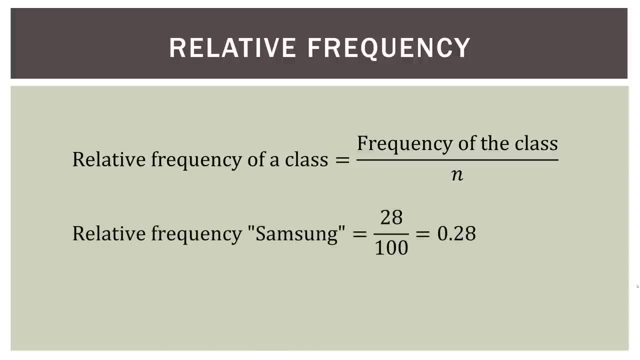 So, for example, in this case, the relative frequency of Samsung is 28 observations out of 100.. So there were 28 people in our data that had a Samsung phone out of 100 people total, and therefore the relative frequency is 0.28. 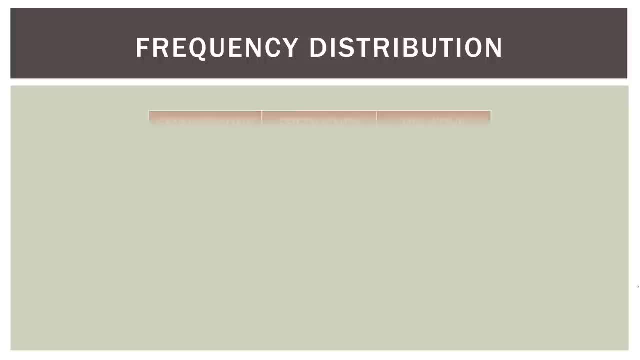 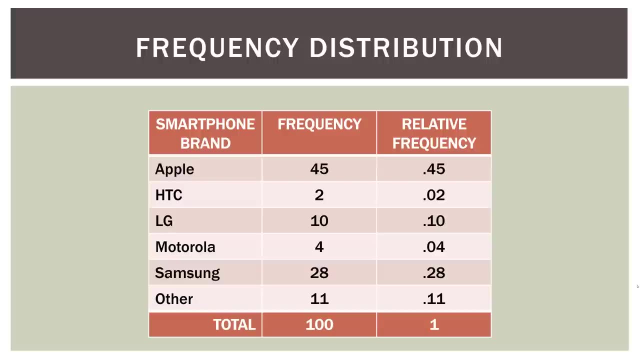 Now we can create a frequency distribution which is very similar to the other chart we created. So here we have our smartphone brand, our frequency- what we did a couple slides ago- and then the relative frequency for each one. Now, I will say that I made this very easy. 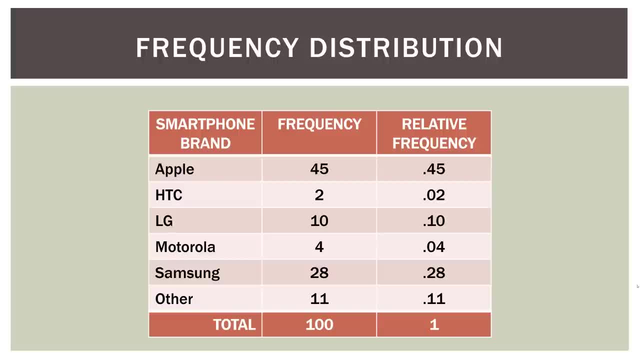 by having 100 observations, but that's not always gonna be the case- Actually, that'll rarely be the case, But still, it's the frequency divided by the total number of observations and that will give you your relative frequency. So in this case- Apple- we had 45 people. 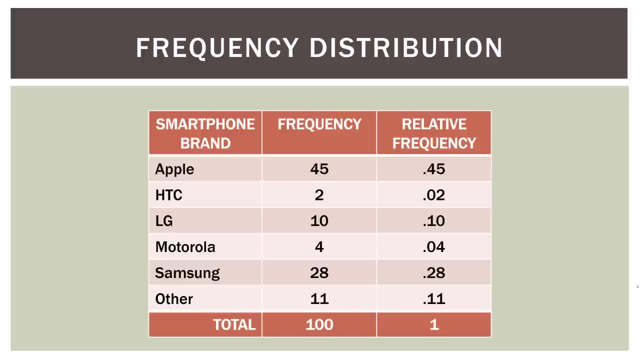 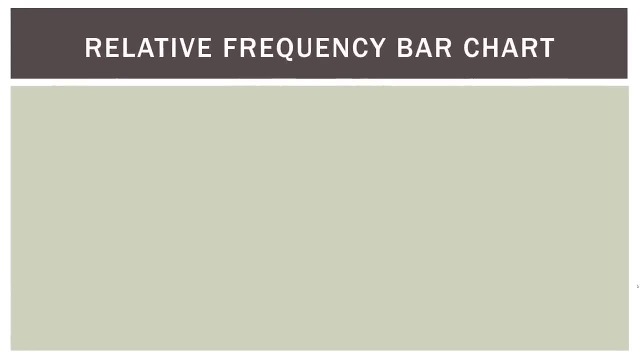 have an Apple phone out of 100.. 45 divided by 100 is 0.45.. And you can see how that goes down the chart Very straightforward. Now we can do the same thing for a frequency bar chart. relative frequency bar chart. 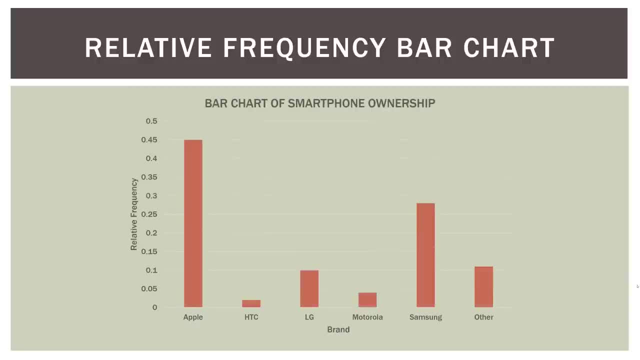 Here it looks exactly the same, except the only difference here is that on the left-hand side, on the y-axis, we have relative frequency instead of the actual frequency or the counts. But the basic idea is the same. Very straightforward, very simple.